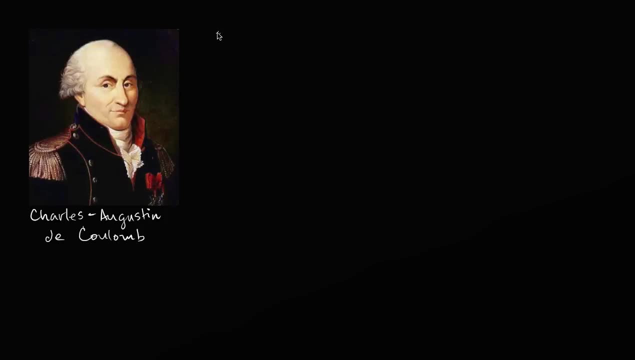 So we've already started to familiarize ourselves with the notion of charge. We've seen that if two things have the same charge- so they're either both positive or they are both negative- then they're going to repel each other. So in either of these cases, 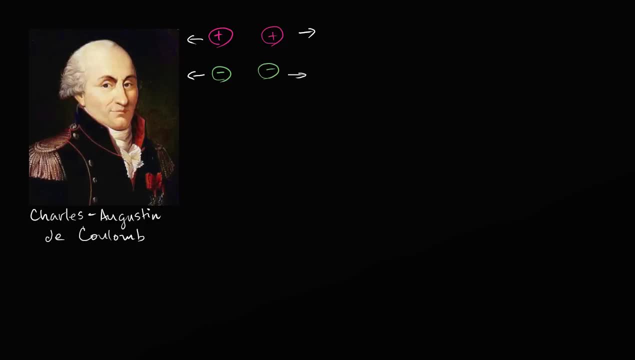 these things are going to repel each other, But if they have different charges, they're going to attract each other. So if I have a positive and I have a negative, they're going to attract each other. This charge is this property of matter. 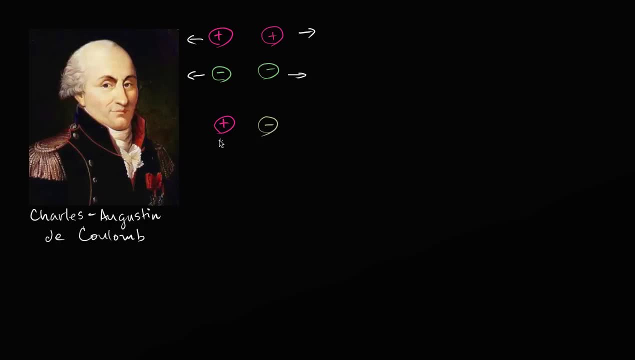 that we've started to observe and we've started to observe of how these different charges, this framework that we've created, how these things start to interact with each other. So these things are going to, these two things are going to attract each other. 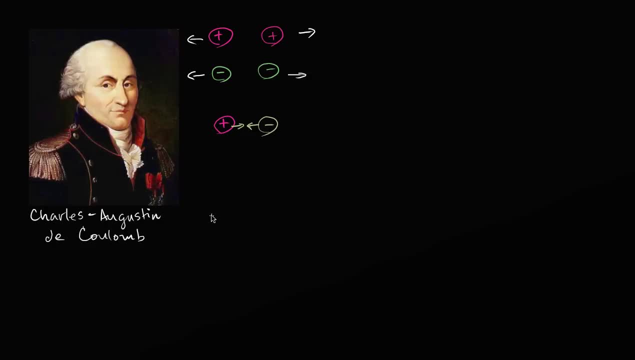 But the question is well, what causes? how can we predict how strong the force of attraction or repulsion is going to be between charged particles- And this was a question- people have noticed, I guess, what you could call electrostatics for a large swath of recorded human history. 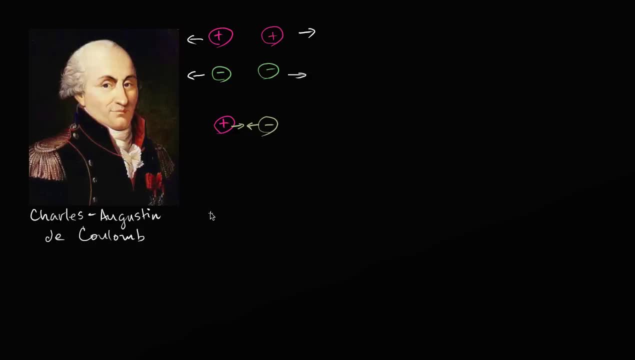 but it wasn't until the 1600s, and especially the 1700s, that people started to seriously view this as something that they could manipulate and even start to predict in a kind of serious mathematical, scientific way, And it wasn't until 1785,. 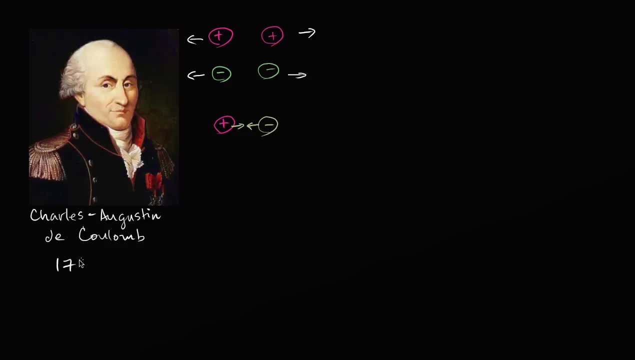 and there were many that came before Coulomb. but in 1785, Coulomb formally published what is known as Coulomb's Law And the purpose of Coulomb's Law. Coulomb's Law is to predict what is going to be the force. 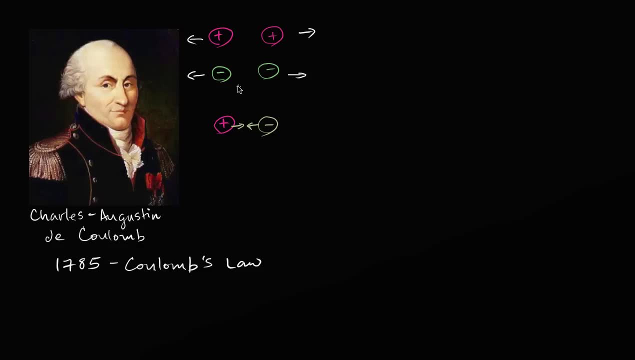 of the electrostatic force of attraction or repulsion between two forces. And so in Coulomb's Law what it states is: is if I have two charges, so let me. so let's say this charge right over here, and I'm going to make it in white. 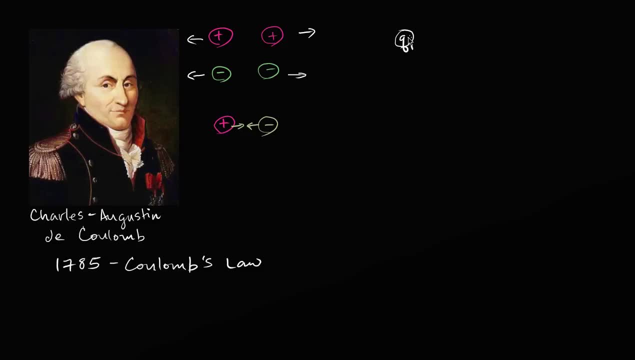 because it could be positive or negative, but I'll just make it Q1,. it has some charge, and then I have in Coulomb's and then another charge, Q2, right over here, another charge, Q2, and then I have the distance. 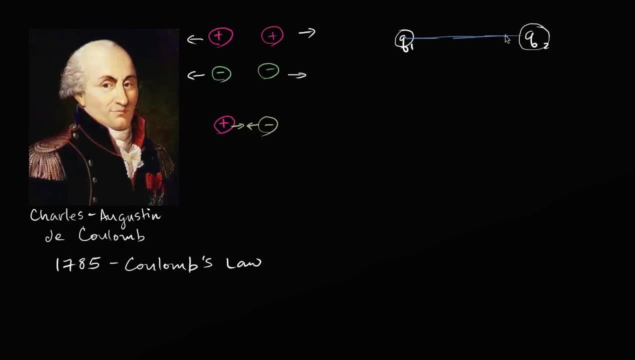 between them being R, so the distance between these two is going to be R. Coulomb's Law states that the force the magnitude of the force, so it could be a repulsive force or it could be an attractive force, which would tell us the direction of the force. 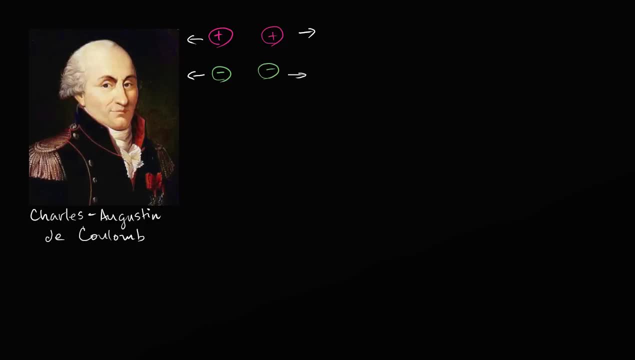 these things are going to repel each other, But if they have different charges, they're going to attract each other. So if I have a positive and I have a negative, they're going to attract each other. This charge is this property of matter. 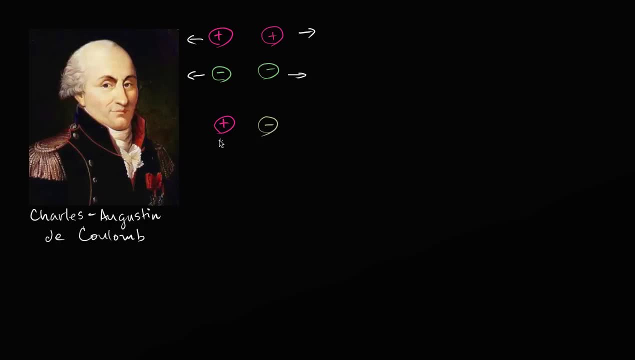 that we've started to observe and we've started to observe of how these different charges, this framework that we've created, how these things start to interact with each other. So these things are going to, these two things are going to attract each other. 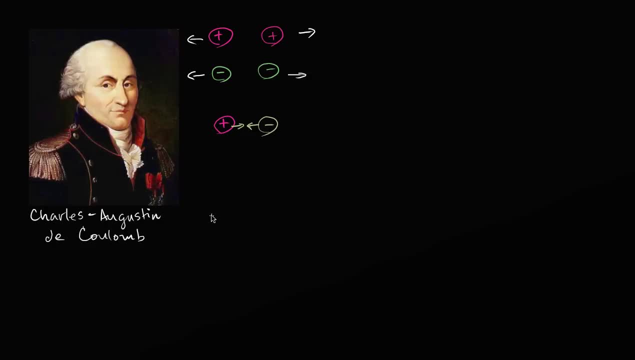 But the question is well, what causes? how can we predict how strong the force of attraction or repulsion is going to be between charged particles- And this was a question- people have noticed, I guess, what you could call electrostatics for a large swath of recorded human history. 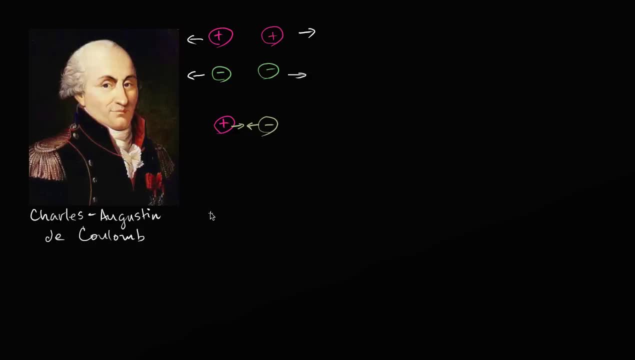 but it wasn't until the 1600s, and especially the 1700s, that people started to seriously view this as something that they could manipulate and even start to predict in a kind of serious mathematical, scientific way, And it wasn't until 1785,. 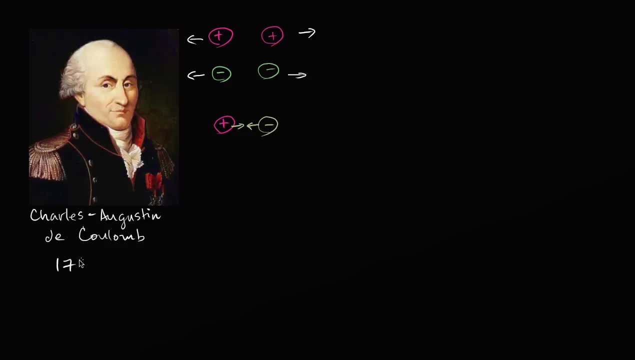 and there were many that came before Coulomb. but in 1785, Coulomb formally published what is known as Coulomb's Law And the purpose of Coulomb's Law. Coulomb's Law is to predict what is going to be the force. 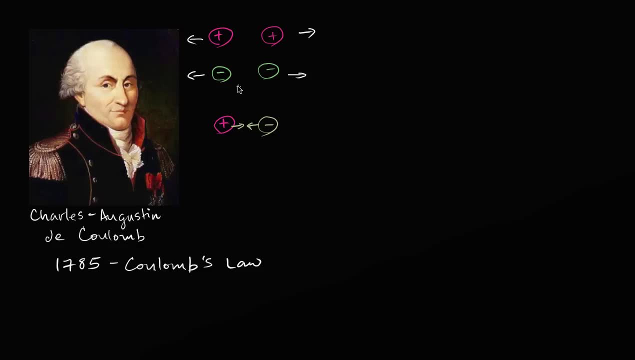 of the electrostatic force of attraction or repulsion between two forces. And so in Coulomb's Law what it states is: is if I have two charges, so let me. so let's say this charge right over here, and I'm going to make it in white. 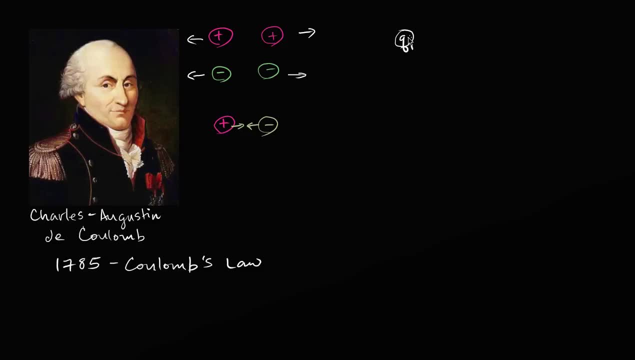 because it could be positive or negative, but I'll just make it Q1,. it has some charge, and then I have in Coulomb's and then another charge, Q2, right over here, another charge, Q2, and then I have the distance. 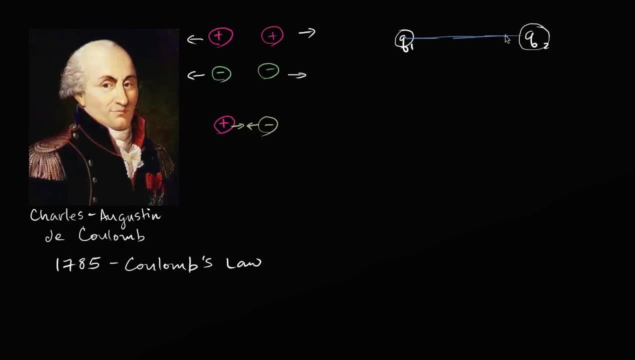 between them being R, so the distance between these two is going to be R. Coulomb's Law states that the force the magnitude of the force, so it could be a repulsive force or it could be an attractive force, which would tell us the direction of the force. 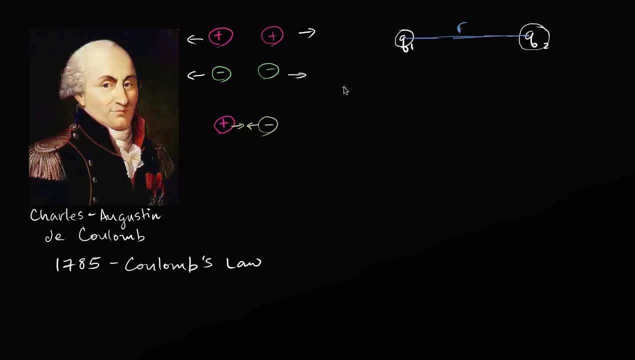 between the two charges, but the magnitude of the force, which I'll just write it as F, the magnitude of the electrostatic force. I'll write the sub-E here, the subscript E for electrostatic Coulomb stated. well, this is going to be. 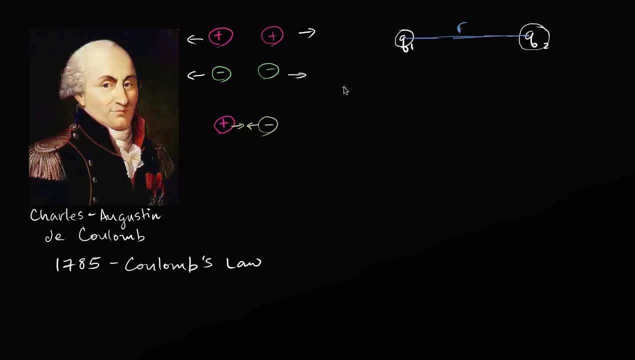 between the two charges, but the magnitude of the force, which I'll just write it as F, the magnitude of the electrostatic force. I'll write the sub-E here, the subscript E for electrostatic Coulomb stated. well, this is going to be. 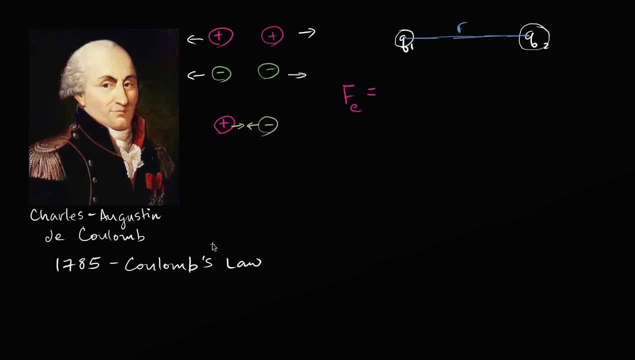 and he tested this. he didn't just kind of guess this. people actually were assuming that it had something to do with the products of the magnitude of the charges and that as the particles got further and further away, the electrostatic force dissipated. 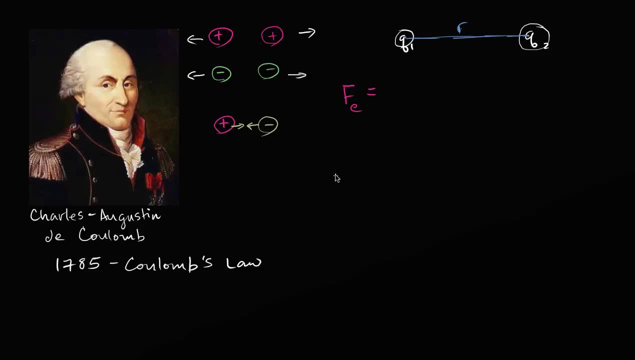 but he was able to actually measure this and feel really good about stating this law. He stated that the magnitude of the electrostatic force is proportional is proportional to the product of the magnitudes of the charges. So I could write this as Q1 times Q. 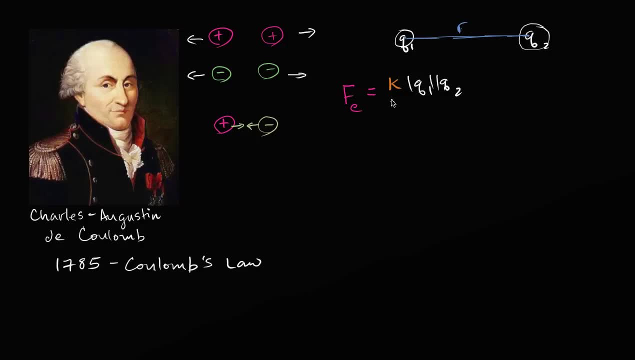 Q2, and I could take the absolute value of each, which is the same thing as just taking the absolute value of the product, And here's why I'm taking the absolute value of the product. Well, if they're different charges, this will be a negative number. 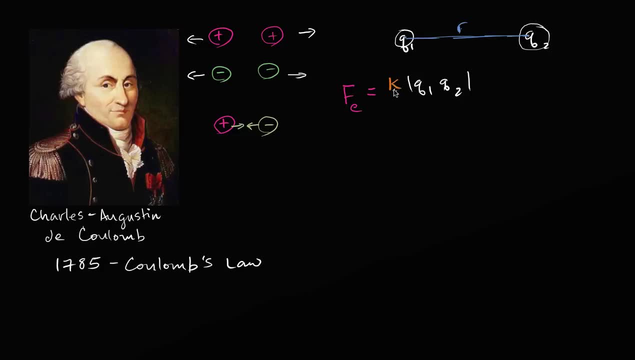 but we just want the overall magnitude of the force. So we could take: it's proportional to the absolute value of the product, of the charges, and it's inversely proportional to not just the distance between them, not just to R, but to the square of the distance. 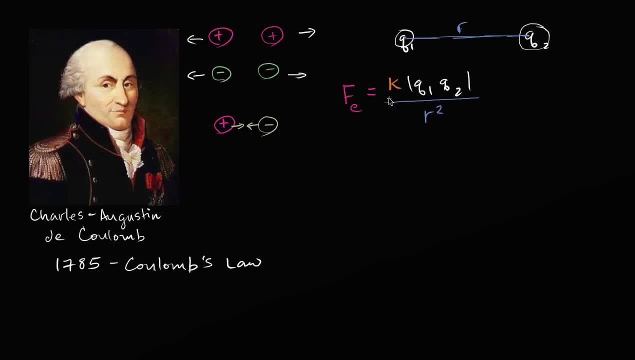 the square of the distance between them. And what's pretty neat about this is how close it mirrors Newton's law of gravitation. Newton's law of gravitation. we know that the force due to gravity between two masses- remember mass- is just another property of matter. 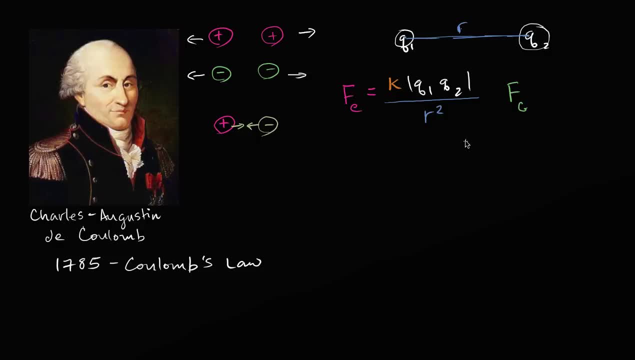 that we sometimes feel is a little bit more tangible, because it feels like, you know, we can kind of see weight and volume, but that's not quite the same, or we can, we feel like we can feel, or internalize things like weight and volume. 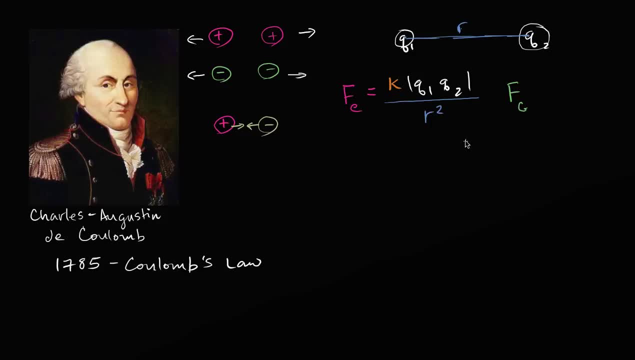 which are related to mass, But in some ways it is just another property, another property, and especially as you get into more kind of fancy physics, our everyday notion of even mass starts to become a lot more interesting. But Newton's law of gravitation says: 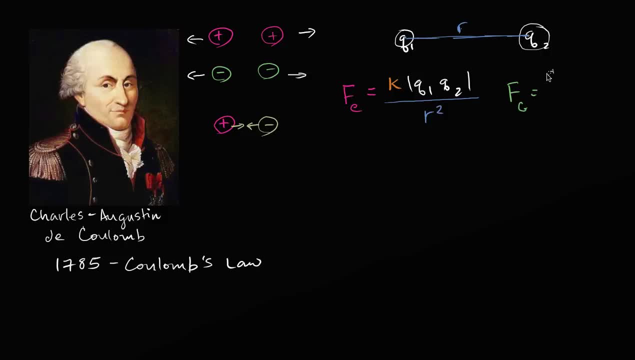 look, the magnitude of the force of gravity between two masses is going to be proportional to by the gravitational constant, proportional to the product of the two masses. Actually, let me do it in those same colors, so you can see the color, so you can see the relationship. 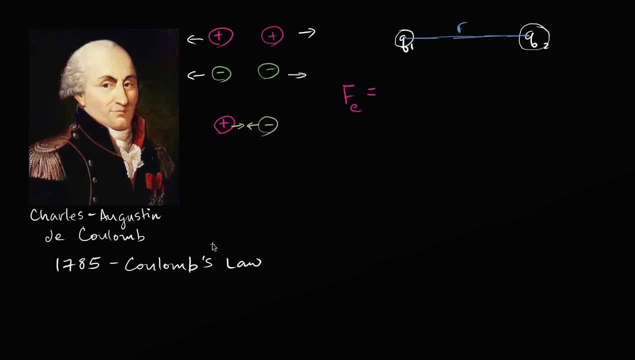 and he tested this. he didn't just kind of guess this. people actually were assuming that it had something to do with the products of the magnitude of the charges and that as the particles got further and further away, the electrostatic force dissipated. 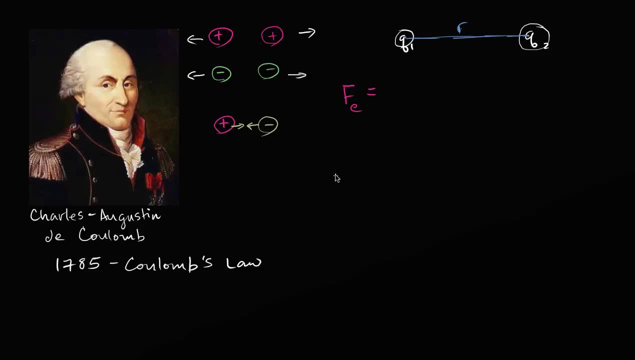 but he was able to actually measure this and feel really good about stating this law. He stated that the magnitude of the electrostatic force is proportional is proportional to the product of the magnitudes of the charges. So I could write this as Q1 times Q. 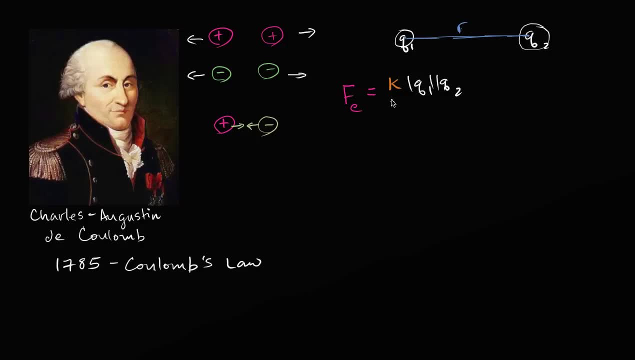 Q2, and I could take the absolute value of each, which is the same thing as just taking the absolute value of the product, And here's why I'm taking the absolute value of the product. Well, if they're different charges, this will be a negative number. 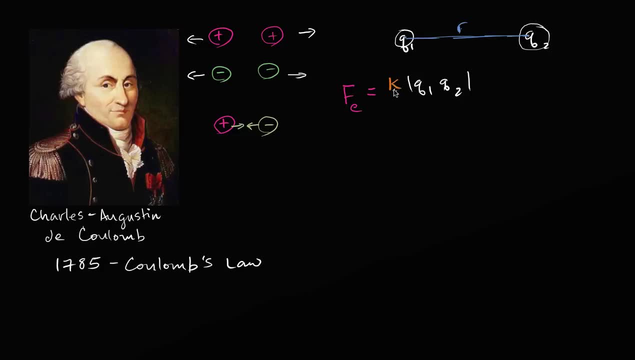 but we just want the overall magnitude of the force. So we could take: it's proportional to the absolute value of the product, of the charges, and it's inversely proportional to not just the distance between them, not just to R, but to the square of the distance. 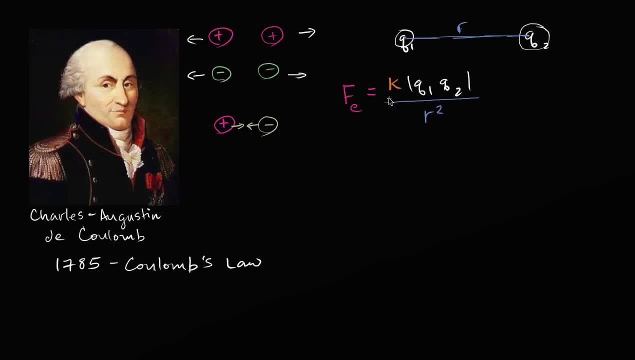 the square of the distance between them. And what's pretty neat about this is how close it mirrors Newton's law of gravitation. Newton's law of gravitation. we know that the force due to gravity between two masses- remember mass- is just another property of matter. 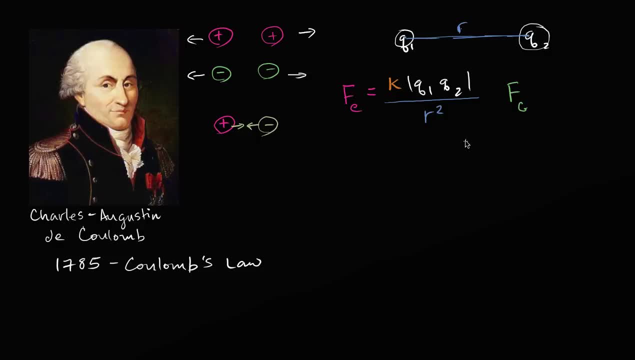 that we sometimes feel is a little bit more tangible, because it feels like, you know, we can kind of see weight and volume, but that's not quite the same, or we can, we feel like we can feel, or internalize things like weight and volume. 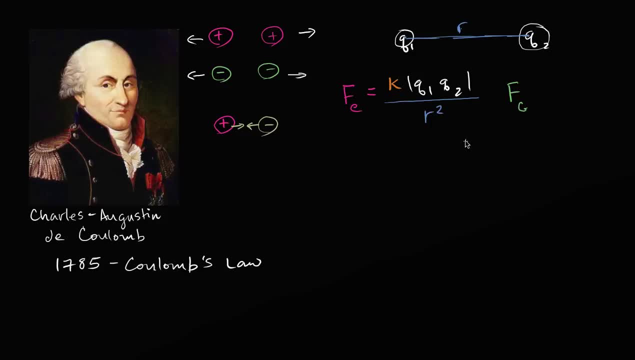 which are related to mass, But in some ways it is just another property, another property, and especially as you get into more kind of fancy physics, our everyday notion of even mass starts to become a lot more interesting. But Newton's law of gravitation says: 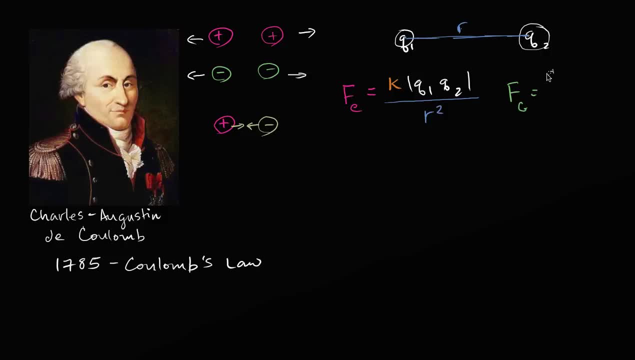 look, the magnitude of the force of gravity between two masses is going to be proportional to by the gravitational constant, proportional to the product of the two masses. Actually, let me do it in those same colors, so you can see the color, so you can see the relationship. 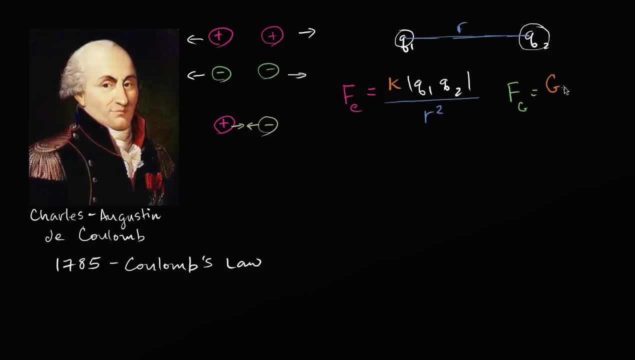 It's going to be proportional to the product of the two masses, m1, m2, and it's going to be inversely proportional to the square of the distance, the square of the distance between two masses. Now, these proportionality constants are very different. 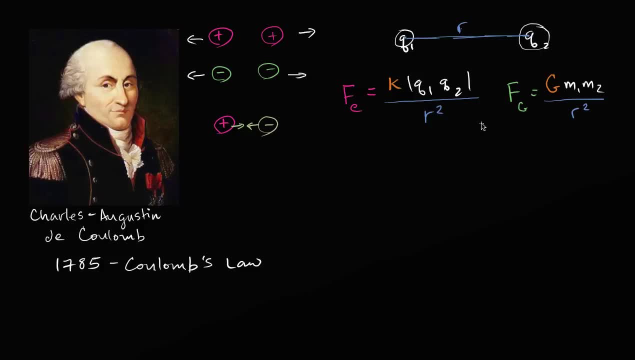 Gravitational force. we kind of perceive this as acting being stronger. it's a weaker force in close range, but we kind of imagine it as kind of what dictates what happens in the amongst the stars and the planets and moons, while the electrostatic force at close range. 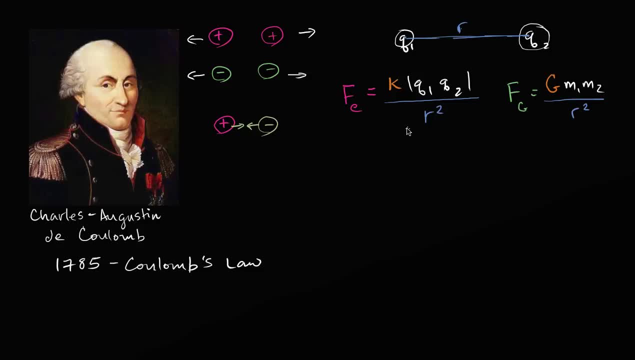 is a much stronger force. it can overcome the gravitational force very easily, but it's what we consider happening at either an atomic level or kind of at a scale that we are more familiar to operating at. But needless to say, it's very interesting. 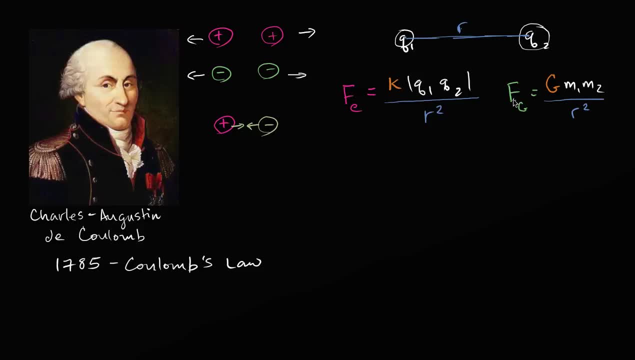 to see how this parallel between these two things. it's kind of these patterns in the universe. But with that said, let's actually apply. let's actually apply Coulomb's Law, just to make sure that we feel comfortable with the mathematics. So let's say that I have a charge here. 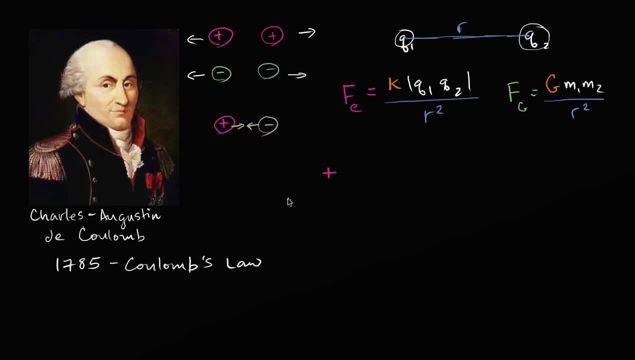 Let's say that I have a charge here and it has a positive charge of I don't know. let's say it is positive five times 10 to the negative three Coulombs. So that's this one right over here, That's its charge. 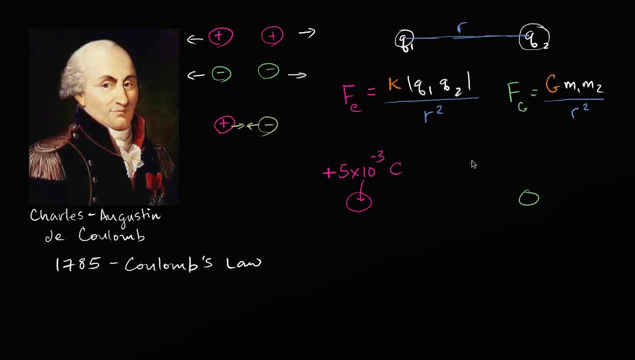 And let's say I have this other charge right over here and this has a negative charge and it is going to be. it is going to be, let's say it's negative one negative one times 10 to the negative one: Coulombs. 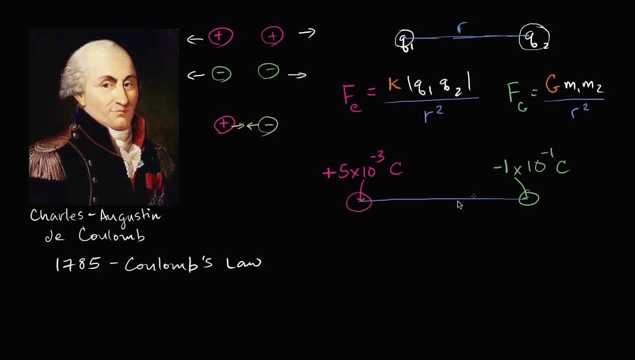 And let's say that the distance between the two, let's say that this distance right here is 0.5 meters. So, given that, let's figure out what the electrostatic force between these two are going to be, And we can already predict that it's going to be. 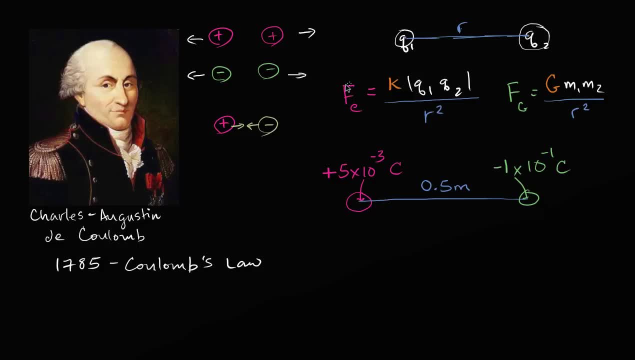 an attractive force because they have different signs, And that was actually part of Coulombs' Law. This is the magnitude of the force. If these have different signs, it's attractive. If they have the same signs, then they are going to repel each other. 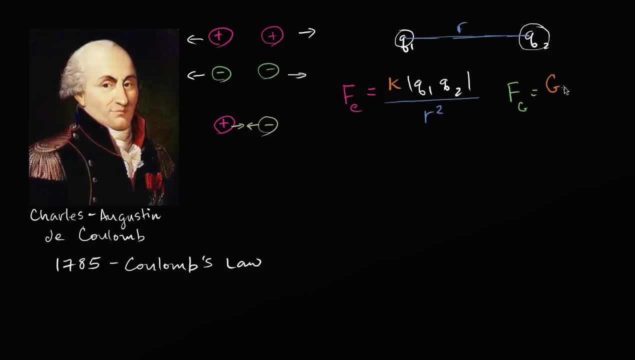 It's going to be proportional to the product of the two masses, m1, m2, and it's going to be inversely proportional to the square of the distance, the square of the distance between two masses. Now, these proportionality constants are very different. Gravitational force. we kind of perceive this as acting being stronger. it's a weaker force in close range, but we kind of imagine it as kind of what dictates what happens in the amongst the stars and the planets and moons, while the electrostatic force at close range. 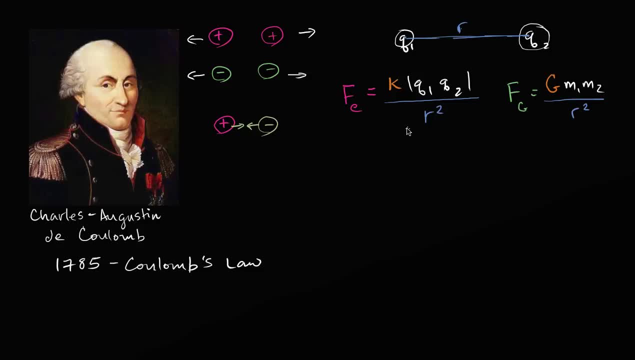 is a much stronger force. it can overcome the gravitational force very easily, but it's what we consider happening at either an atomic level or kind of at a scale that we are more familiar to operating at. But needless to say, it's very interesting. 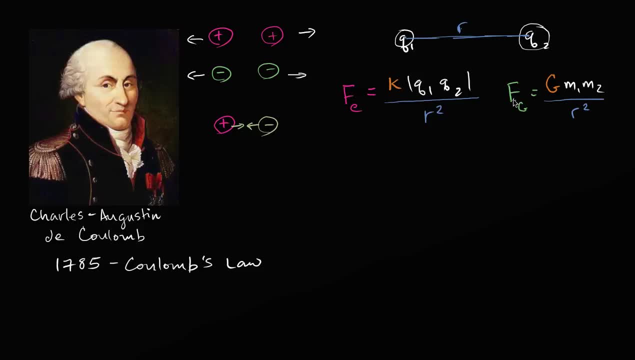 to see how this parallel between these two things. it's kind of these patterns in the universe. But with that said, let's actually apply. let's actually apply Coulomb's Law, just to make sure that we feel comfortable with the mathematics. So let's say that I have a charge here. 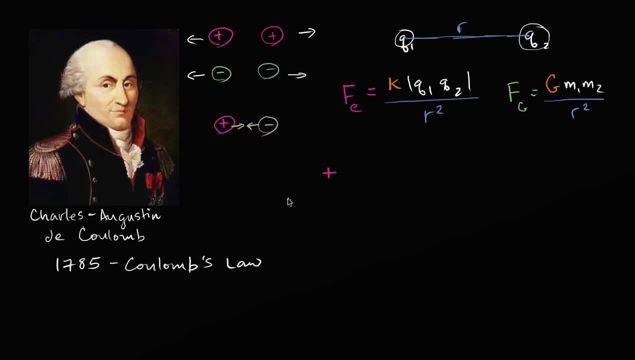 Let's say that I have a charge here and it has a positive charge of I don't know. let's say it is positive five times 10 to the negative three Coulombs. So that's this one right over here, That's its charge. 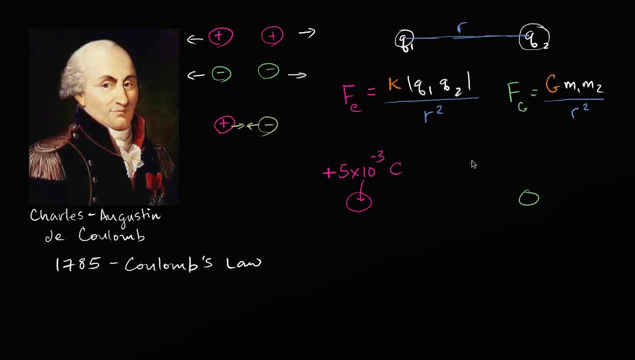 And let's say I have this other charge right over here and this has a negative charge and it is going to be. it is going to be, let's say it's negative one negative one times 10 to the negative one: Coulombs. 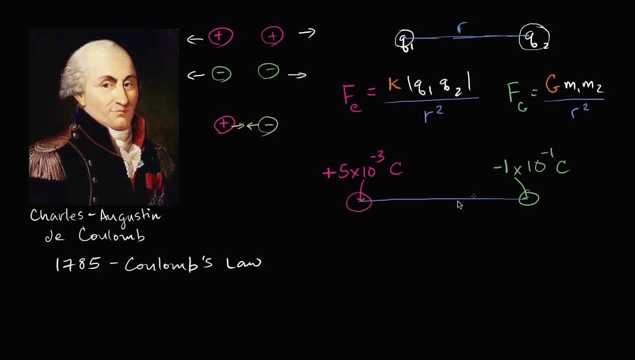 And let's say that the distance between the two, let's say that this distance right here is 0.5 meters. So, given that, let's figure out what the electrostatic force between these two are going to be, And we can already predict that it's going to be. 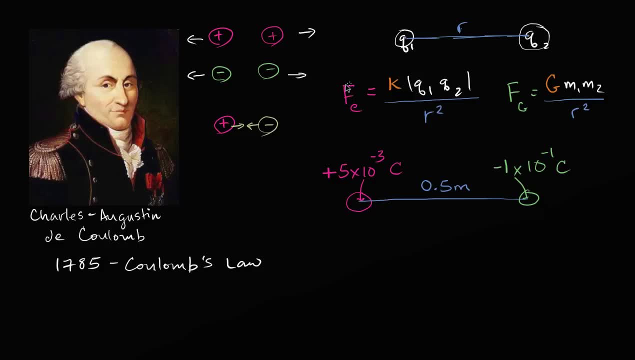 an attractive force because they have different signs, And that was actually part of Coulombs' Law. This is the magnitude of the force. If these have different signs, it's attractive If they have the same signs, it's attractive If they have different signs. 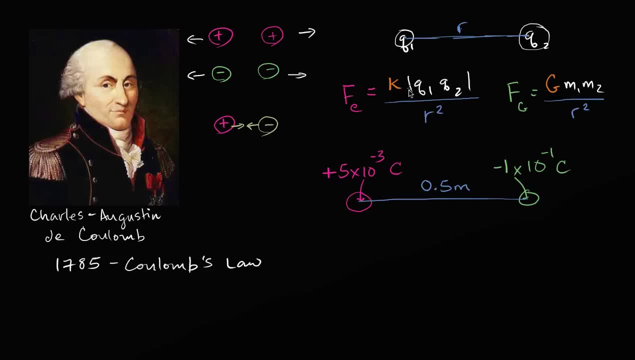 then they are going to repel each other, And I know what you're saying. Well, in order to actually calculate it, I need to know what K is. What is this electrostatic constant? what is this electrostatic constant going to actually be? 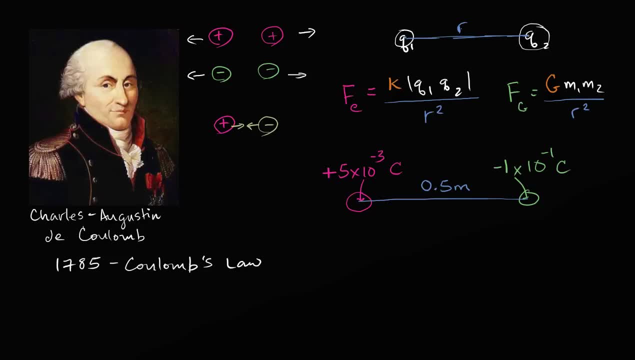 And I know what you're saying. Well, in order to actually calculate it, I need to know what K is, What is this electrostatic constant, what is this electrostatic constant going to actually be, And so you can measure that with a lot of precision. 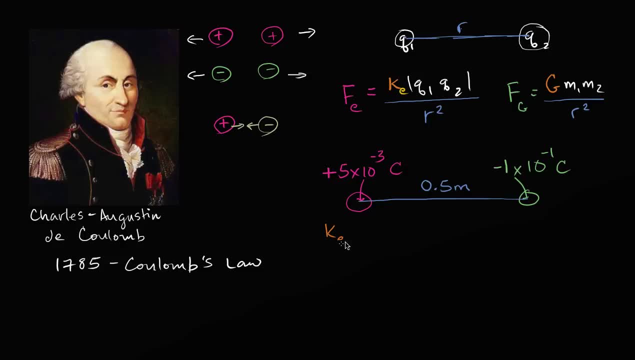 and we have kind of modern numbers on it. But the electrostatic constant, especially for the sake of this problem, I mean, if we were to get really precise, it's 8.987551,. we could keep going on and on. 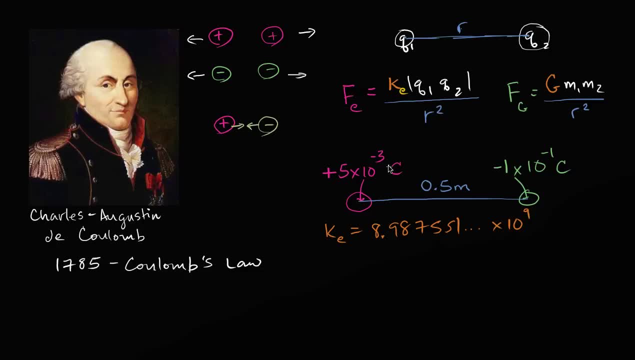 times 10 to the ninth. But for the sake of our little example here, where we really only have one significant digit for each of these, let's just get an approximation. It'll make the math a little bit easier. I won't have to get a calculator out. 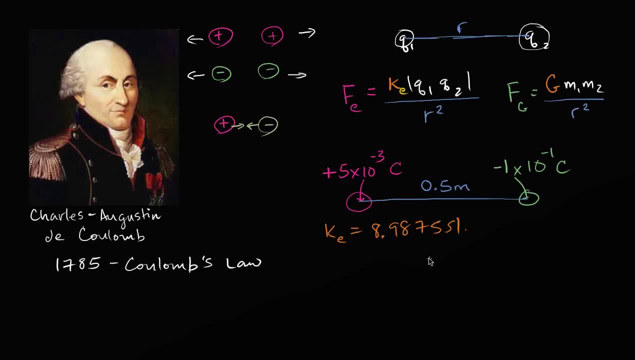 Let's just say it's approximately nine times 10 to the ninth, Nine times 10 to the ninth, Nine times actually. let me make sure it says approximately, because I am approximating here Nine times 10 to the ninth. And what are the units going to be? 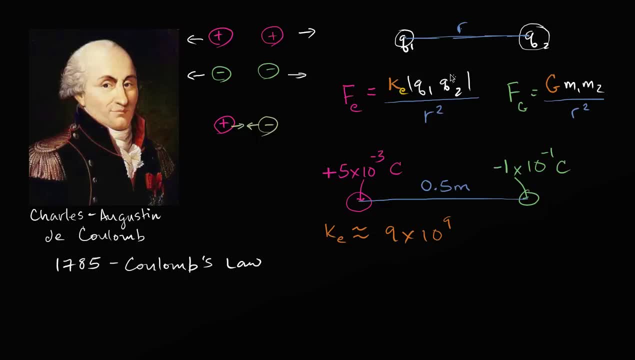 Well, in the numerator here, when I multiply coulombs times coulombs, I'm going to get coulombs squared. This right over here is going to give me that's going to give me coulombs squared, And this down over here is going to give me meters squared. 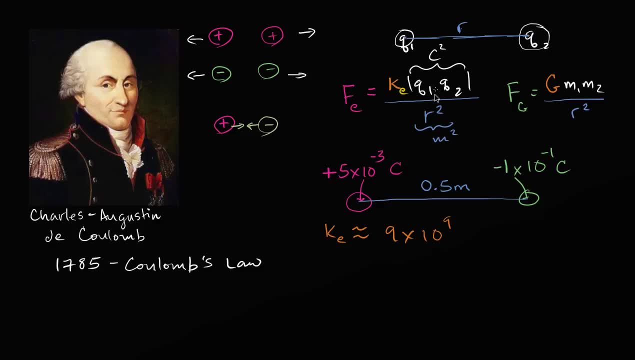 This is going to give me meters squared, And what I want is to get rid of the coulombs and the meters and end up with just the newtons. And so the units here are actually. the units here are newtons, newton and then meters squared. 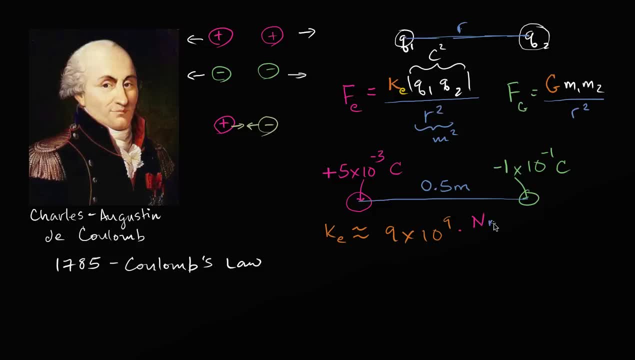 and that cancels out with the meters squared in the denominator Newton, meters squared over coulombs squared, Over over coulombs squared. Let me do that in white: Over over coulombs squared. So these meters squared will cancel with those. 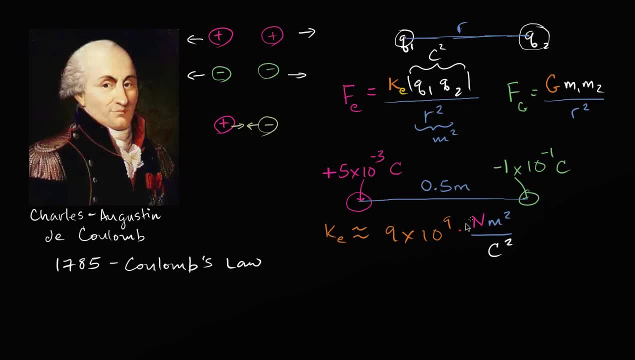 Those coulombs squared in the denominator over here will cancel with those and you'll be just left with newtons. But let's actually do that. Let's actually apply it to this example. I encourage you to pause the video and apply this information to coulombs law. 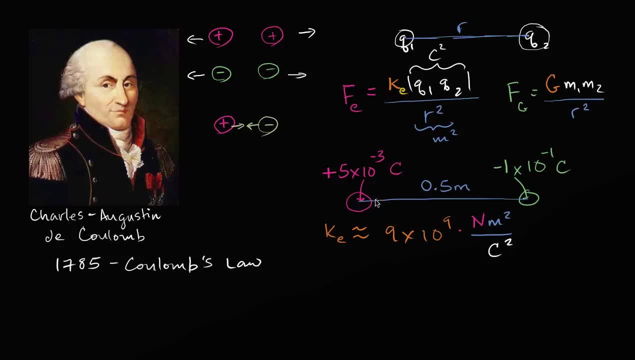 and figure out what the electrostatic force between these two particles is going to be. So I'm assuming you've had your go at it. So it is going to be- and this is really just applying the formula- it's going to be nine times 10 to the ninth. 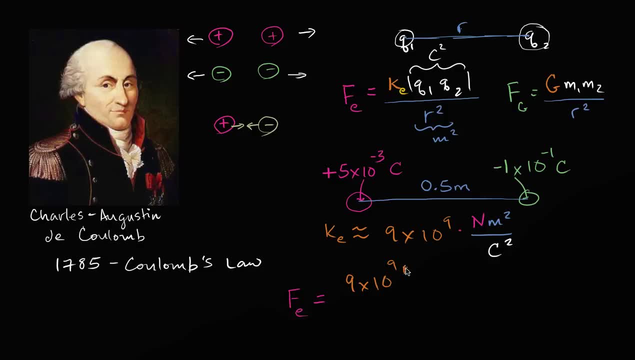 Nine times 10 to the ninth. And I'll write the units here: Newtons, meters squared over coulombs squared, And then q1 times q2.. So this is going to be. let's see, this is going to be. 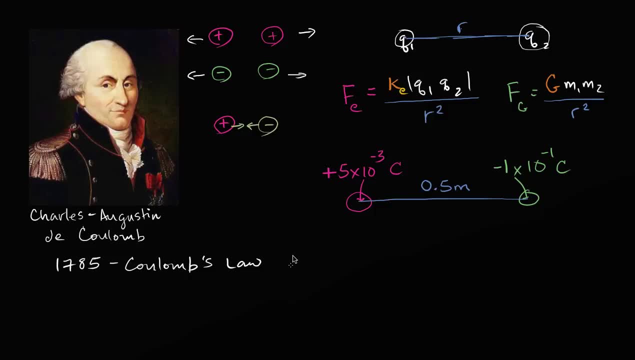 And so you can measure that with a lot of precision and we have kind of modern numbers on it. But the electrostatic constant- especially for the sake of this problem, I mean, if we were to get really precise- it's 8.987551.. 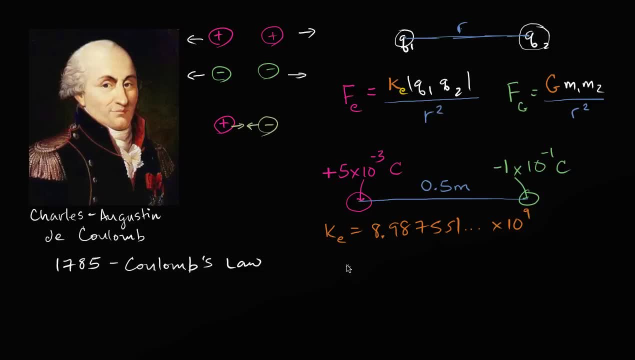 We could keep going on and on times 10 to the ninth. But for the sake of our little example here, where we really only have one significant digit for each of these, let's just get an approximation. It'll make the math a little bit easier. 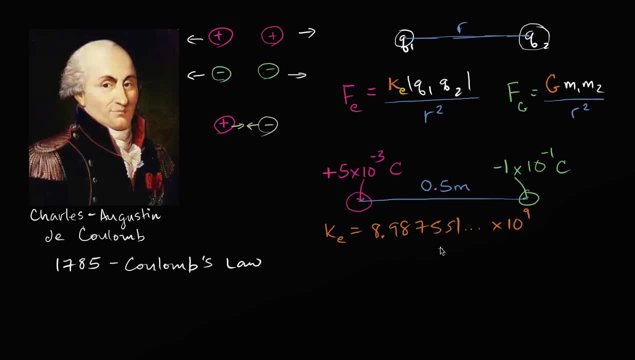 I won't have to get a calculator out. Let's just say it's approximately nine times 10 to the ninth Nine times 10 to the ninth Nine times. actually, let me make sure it says approximately, because I am approximating here. 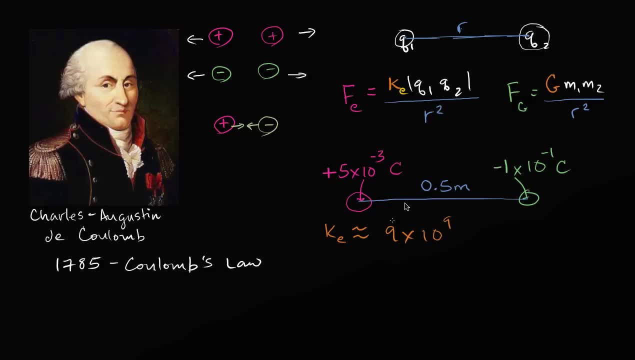 Nine times 10 to the ninth, And what are the units going to be? Well, in the numerator here, if I multiply coulombs times coulombs, I'm going to get coulombs squared. This right over here is going to give me. 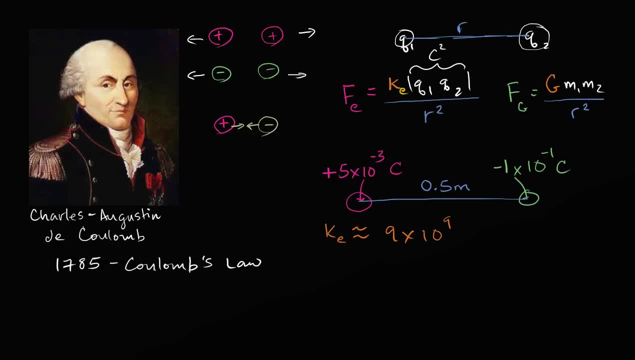 that's going to give me coulombs squared And this down over here is going to give me meters squared. This is going to give me meters squared, And what I want is to get rid of the coulombs and the meters and end up with just the newtons. 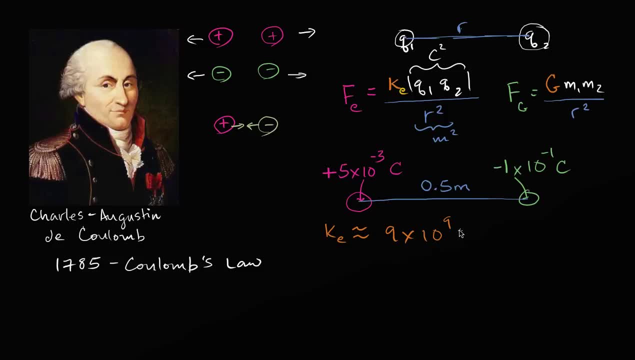 And so the units here are actually the units here are newtons, Newton and then meters squared, and that cancels out with the meters squared in the denominator, Meters squared over coulombs squared Over over coulombs squared. 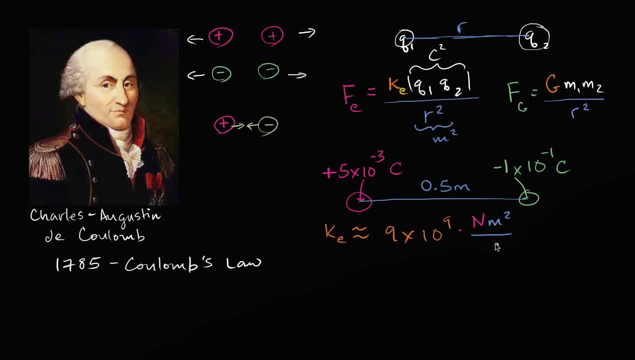 Let me do that in white, Over over coulombs squared. So these meters squared will cancel with those. Those coulombs squared in the denominator over here will cancel with those and you'll be just left with newtons. But let's actually do that. 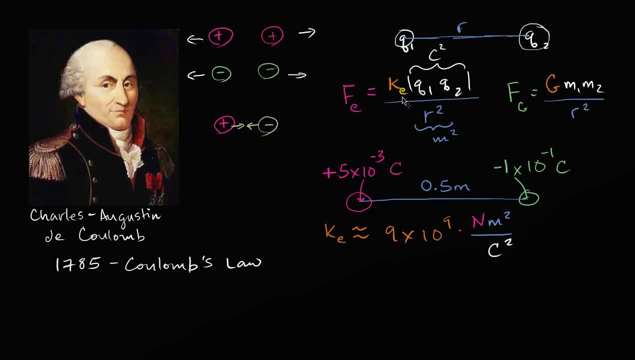 Let's actually apply it to this example. I encourage you to pause the video and apply this information to coulombs law and figure out what the electrostatic force between these two particles is going to be. So I'm assuming you've had your go at it. 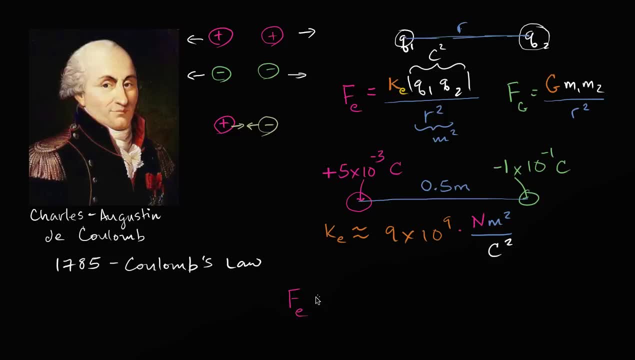 So it is going to be- and this is really just applying the formula- it's going to be nine times 10 to the ninth, Nine times 10 to the ninth. And I'll write the units here: Newtons. meters squared over coulombs squared. 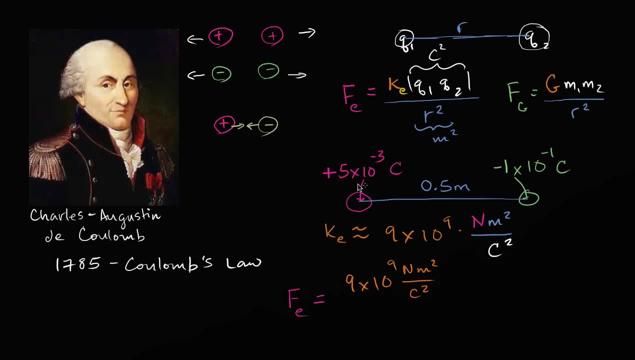 And then Q1 times Q2.. So this is going to be. let's see this is going to be actually. let me just write it all out for this first time. So it's going to be times five times 10 to the negative 30 coulombs. 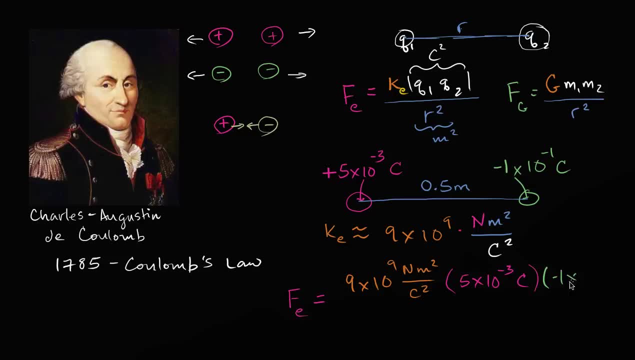 times negative, one times 10 to the negative one, coulombs, And we're going to take the absolute value of this so that negative is going to go away. All of that over, all of that over, we're in kind of the home stretch right over here. 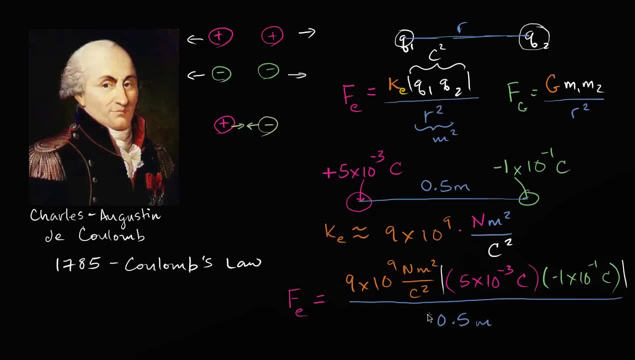 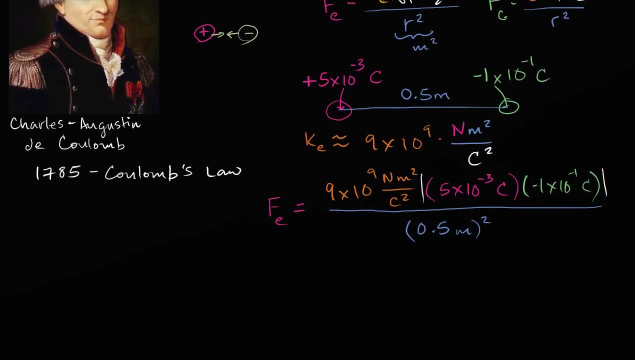 0.5 meters squared. 0.5 meters squared, And so let's just do a little bit of the math here. So first of all let's look at the units. So we have coulombs squared here and then we're going to have coulombs times, coulombs there. 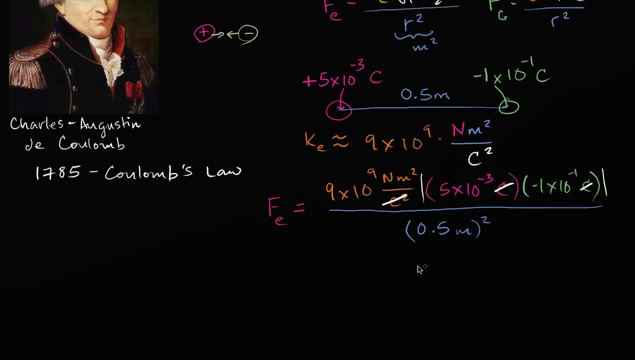 So that's coulombs squared divided by coulombs squared. That's going to cancel with that and that You have meters squared here And actually let me just write it out. So the numerator in the numerator we are going to have, 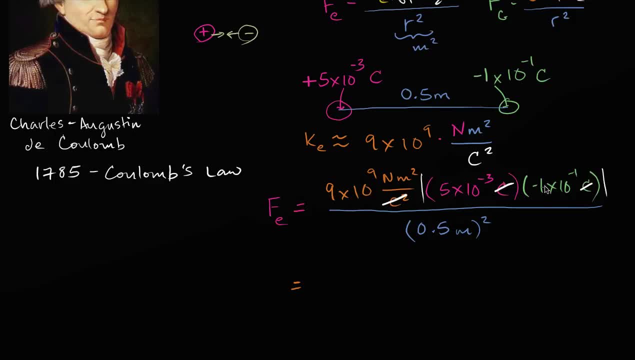 so if we just say nine times five times, well, we take the absolute value, it's just going to be one. So nine times five is going to be nine times five times negative, five times negative. one is negative five with the absolute value there. 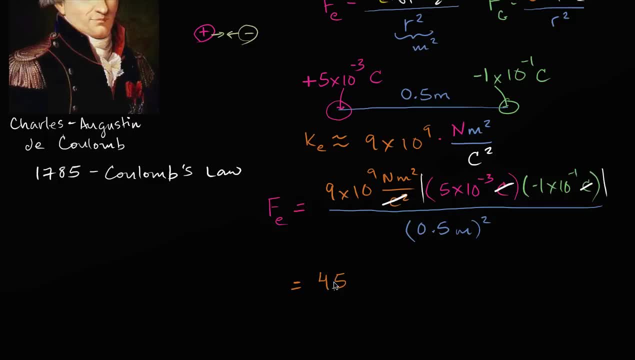 So it's just going to be five times nine. It's gonna be 45 times 10 to the nine, minus three minus one. So six, five. so that's gonna be 10 to the fifth, 10 to the fifth. the Coulomb's already canceled out. 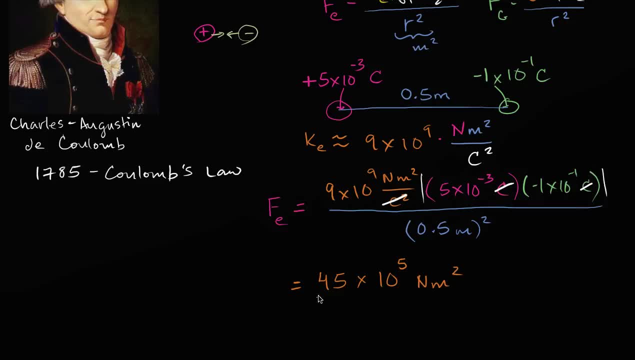 and we're going to have Newton meter squared over, over 0.25 meter squared, 0.25 meter squared. these cancel, And so we are left with: well, if you divide by 0.25, that's the same thing as dividing by 1. fourth, 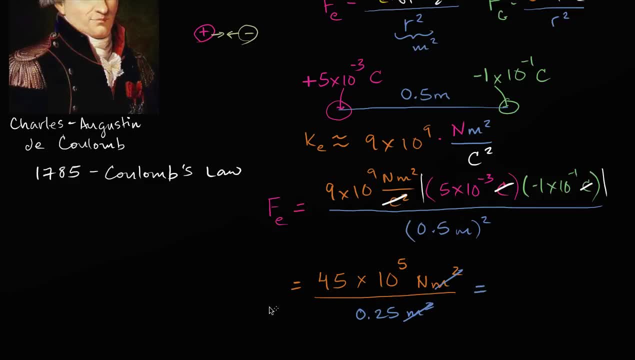 which is the same thing as multiplying by four. So if you multiply this times four, 45 times four, is 160 plus 20, is equal to 180 times 10 to the fifth Newtons. And if we wanted to write it in scientific notation, 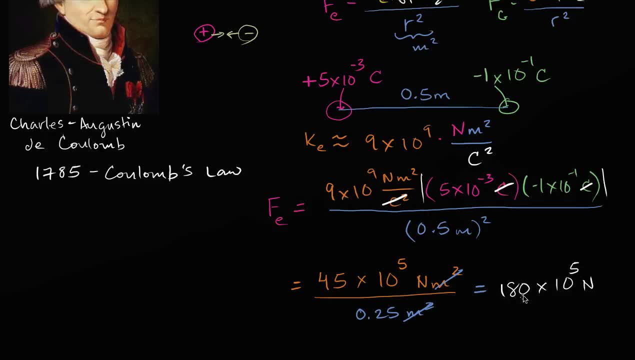 well, we could divide this by. we could divide this by: divide this by 100 and then multiply this by 100, and so you could write this as 1.80 times one point, and actually I don't want to make it look like. 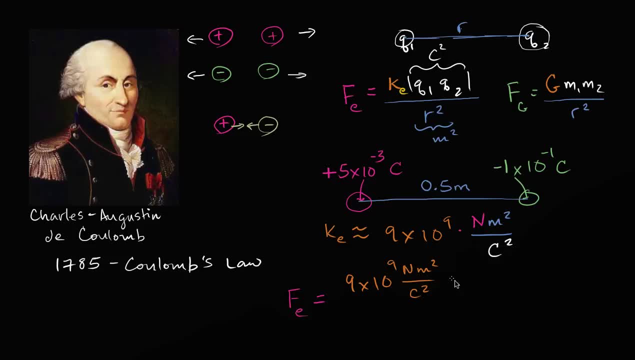 actually, let me just write it all out for this first time. So it's going to be times five times 10 to the negative 30 coulombs, times negative one times 10 to the negative one coulombs, And we're going to take the absolute value of this. 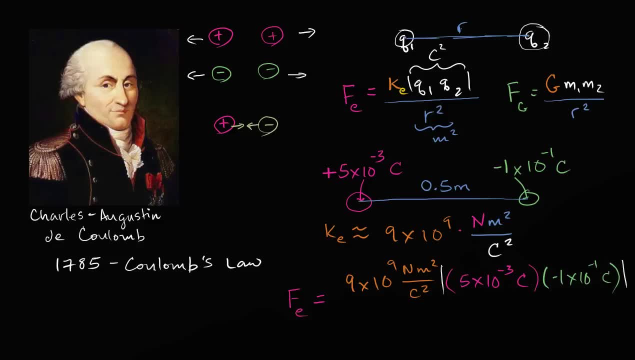 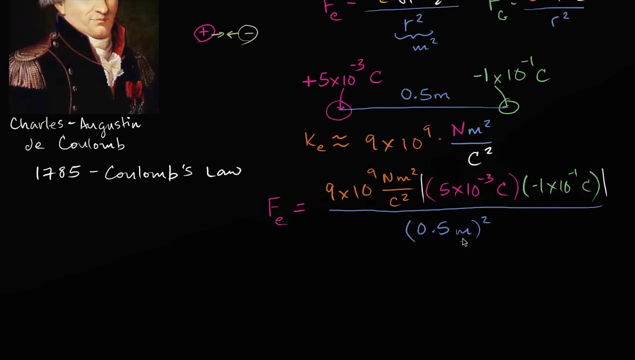 so that negative is going to go away. All of that over. we're in kind of the home stretch right over here, 0.5 meters squared, And so let's just do a little bit of the math here. So first of all let's look at the units. 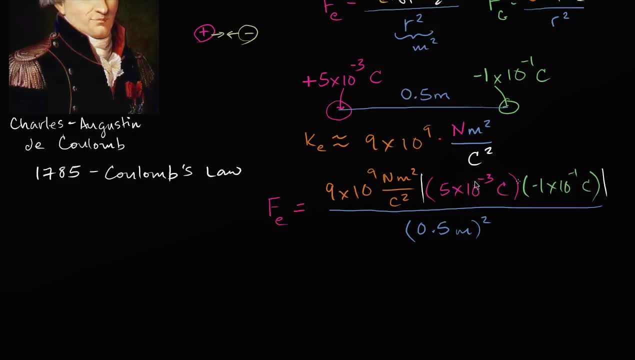 So we have coulombs squared here And then we're going to have coulombs times coulmbs there, That's coulombs squared divided by coulombs squared. That's going to cancel with that and that You have meters squared here. 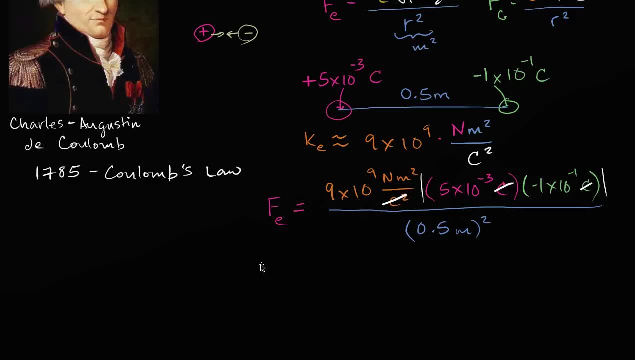 And actually let me just write it out. So in the numerator we are going to have, so if we just say nine times five times, when we take the absolute values, it's going to be one. So nine times five is going nine times, five times negative one. 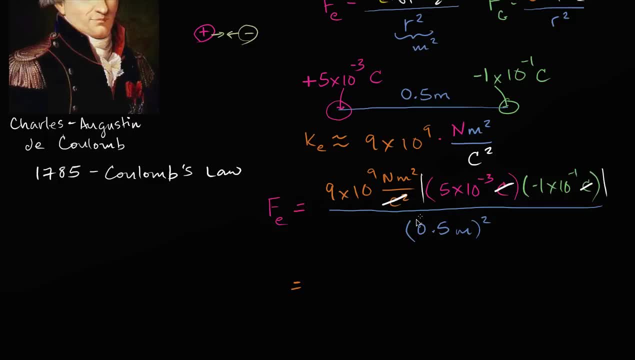 Five times negative. one is negative five, with the absolute value there. So this is going to be five times nine, So it's going to be 45. times 10 to the nine, minus three minus one, So six, five. so that's gonna be 10 to the fifth. 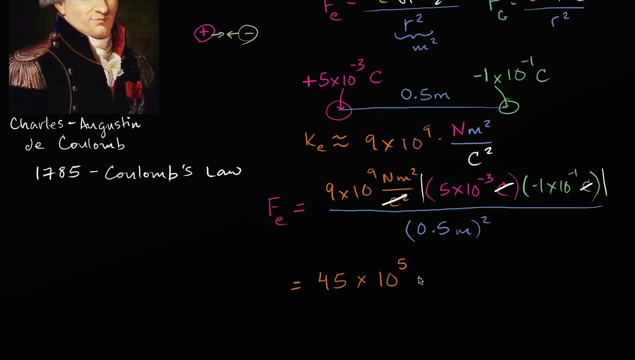 10 to the fifth, the Coulomb's already canceled out and we're going to have Newton meter squared over over 0.25 meter squared. These cancel and so we are left with: well, if you divide by 0.25,. 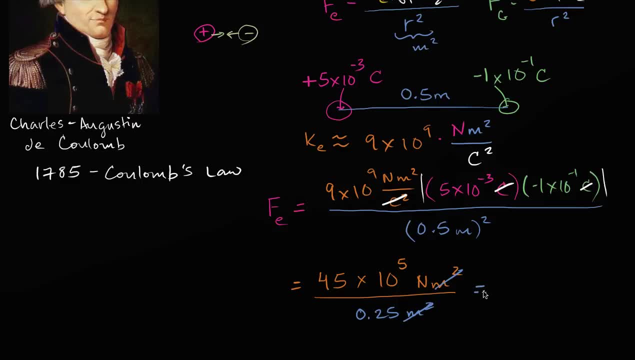 that's the same thing as dividing by 1 fourth, which is the same thing as multiplying by four. So if you multiply this times four, 45 times four is 160 plus 20 is equal to 180 times 10 to the fifth Newtons. 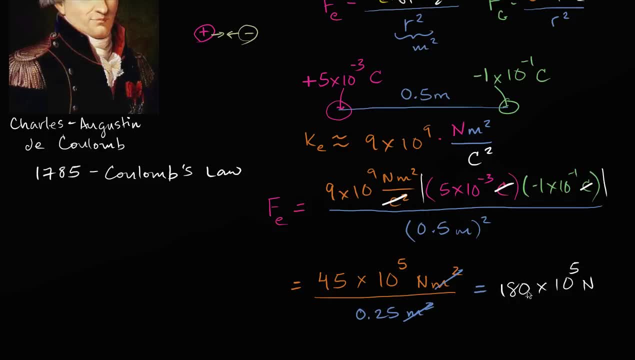 And if we wanted to write it in scientific notation, well, we could divide this by. we could divide this by 100, and then multiply this by 100, and so you could write this as 1.85.. So 1.80 times one point. 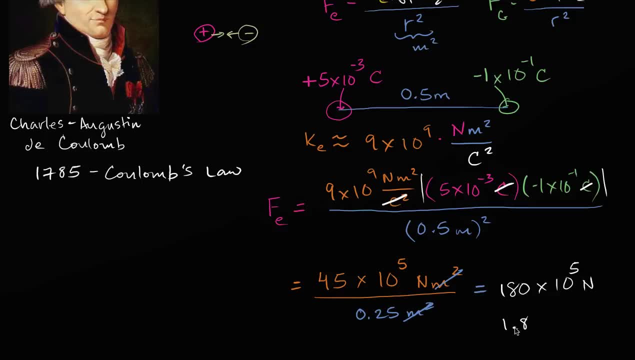 and actually I don't want to make it look like I have more significant digits than I really have: 1.8 times 10 to the seventh times 10 to the seventh Newtons. I just divided this by 100 and I multiplied this by 100..